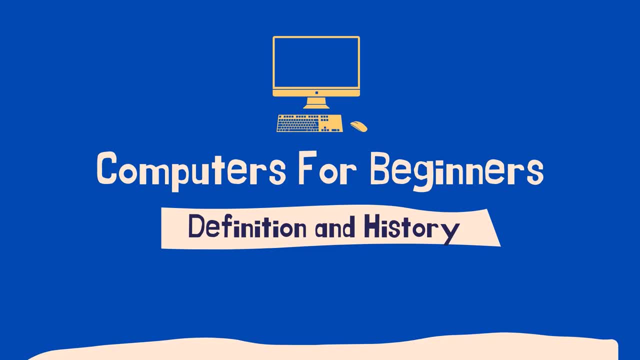 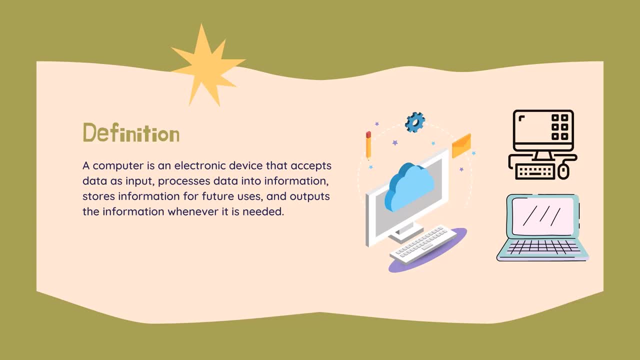 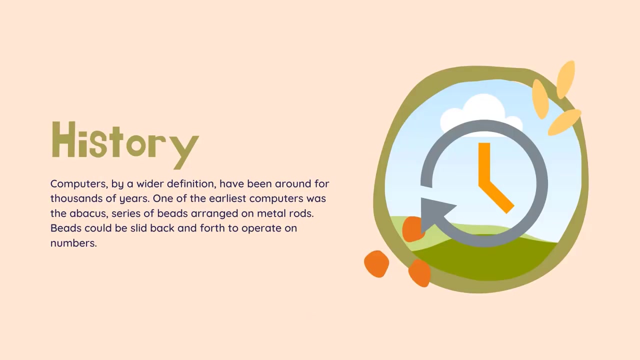 What is a computer? A computer is an electronic device that accepts data as input, processes data into information, stores information for future uses and outputs the information whenever it is needed. Computers, by a wider definition, have been around for thousands of years. 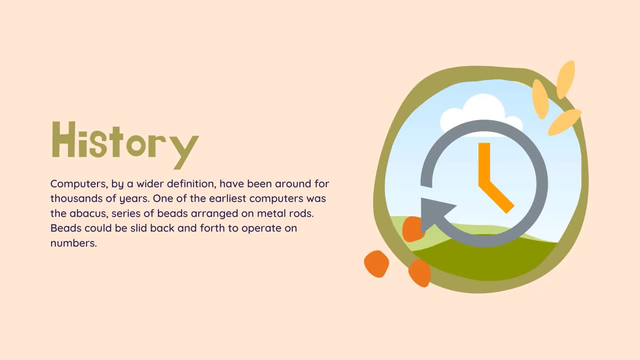 One of the earliest computers was the abacus, series of beads arranged on metal rods. Beads could be slid back and forth to operate on numbers. This was a very rudimentary device and is not commonly thought of as a computer. in modern times, Our idea of computers involves 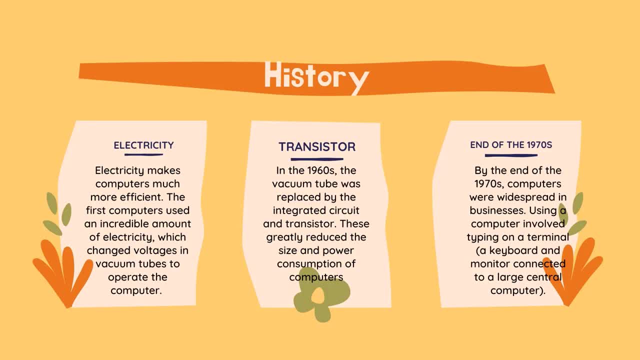 electricity and electronics. Electricity makes computers much more efficient. The first computers used an incredible amount of electricity which changed voltages in vacuum tubes to operate the computer. These computers were given instructions using punch cards and were behemoths taking up entire floors of buildings, Only the more privileged universities and government facilities. 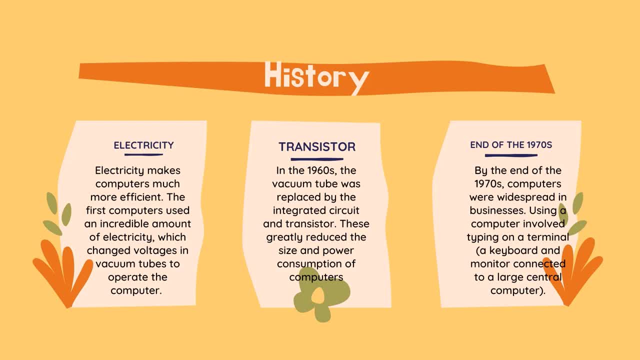 had access to them. In the 1960s, the vacuum tube was replaced by the integrated circuit and transistor. These greatly reduced the size and power consumption. They were still very large by today's standards, but more institutions had access to computing power than ever before. At the end of the decade, the microchip was invented, which reduced the size. 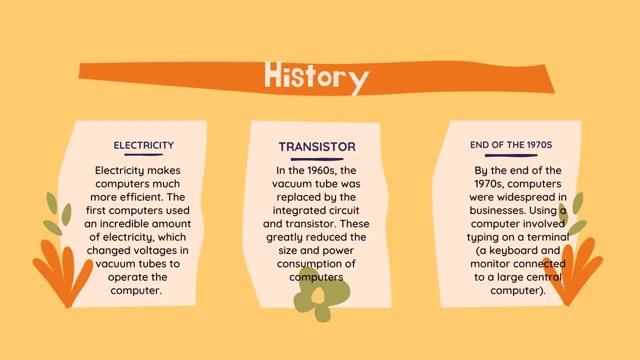 of the computer even more. By the end of the 1970s, computers were widespread in businesses. Using a computer involved typing on a terminal, a keyboard and monitor connected to a large central computer. Soon power was used to power a computer. The computer was used to power a computer. 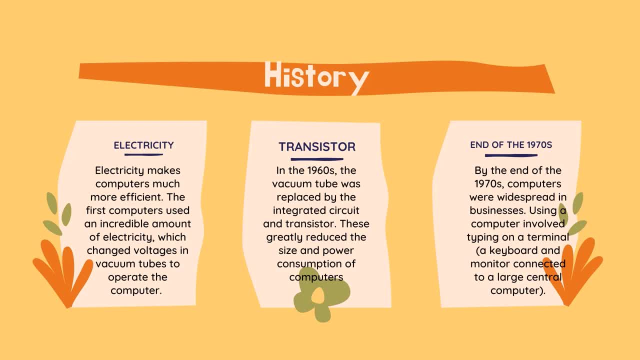 and a computer was used to power a computer, The parts became small enough to allow many users to have a computer at their home. Thus the personal computer, or PC, was born. Since then, personal computers have become tremendously more efficient. They are much smaller and yet have seen extreme. 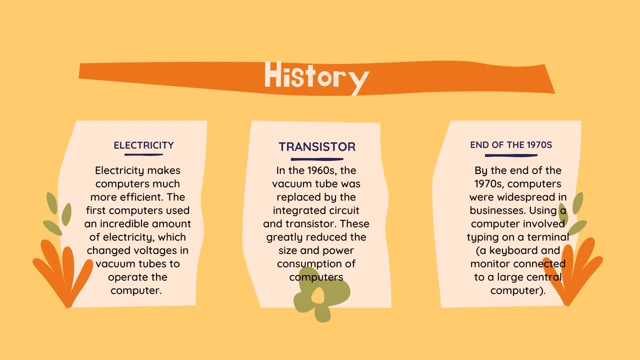 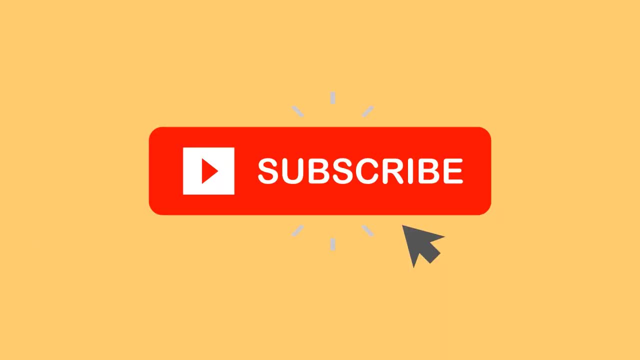 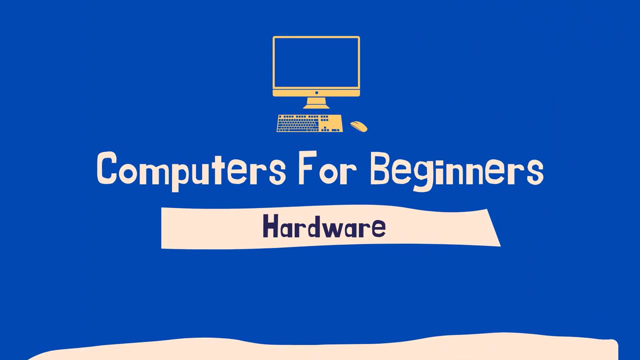 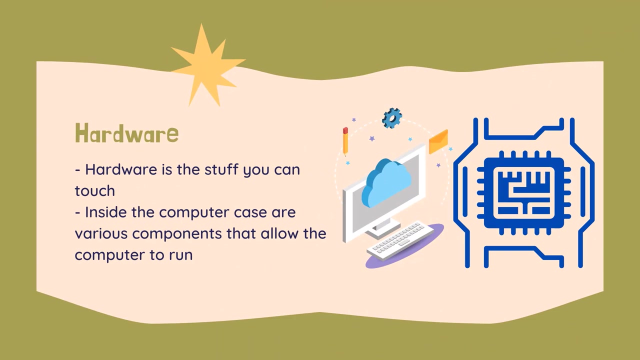 performance gains. In addition to these improvements, computers have become affordable enough for many families worldwide. Hardware is the stuff you can touch, as opposed to software, which is abstract and exists only in a virtual world. as computer code, Hardware is made of materials found in the universe. 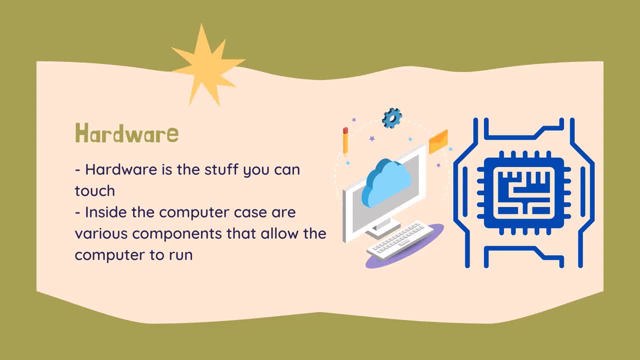 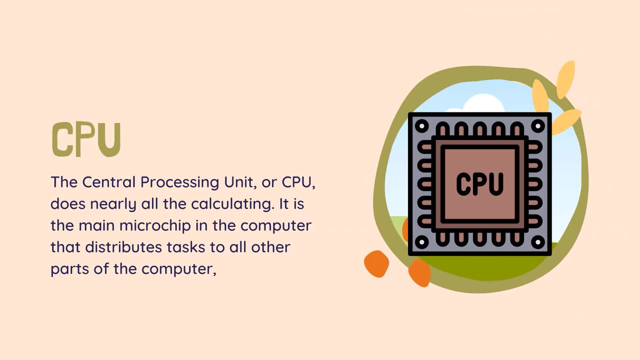 and are subject to the laws of physics. Inside the computer case are various components that allow the computer to run. CPU. the central processing unit, or CPU, does nearly all the calculating. It is the main microchip in the computer that distributes tasks to all other parts of the computer, When most people talk about the processor or chip. 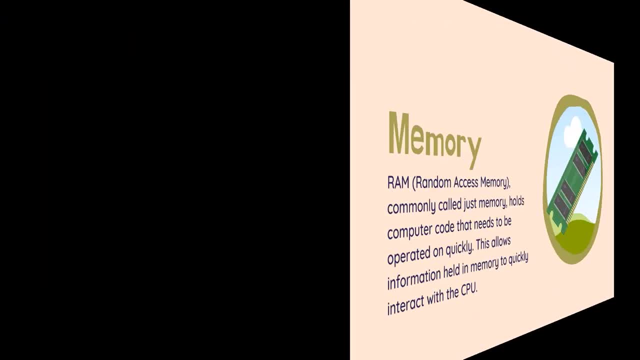 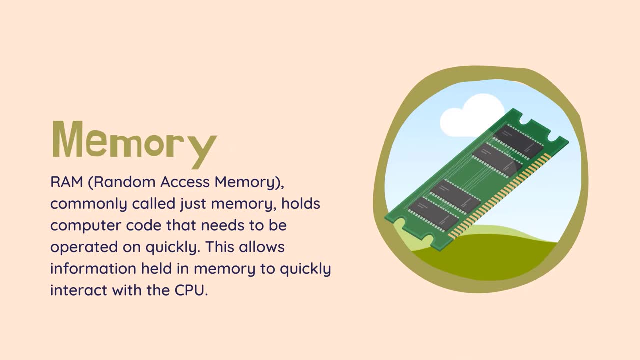 it is actually the CPU. they are referring to RAM. Random Access Memory, commonly called just memory, holds computer code that needs to be operated on quickly. This allows information held in memory to quickly interact with the CPU. The amount of RAM available is limited and therefore needs to be constantly cleared, and 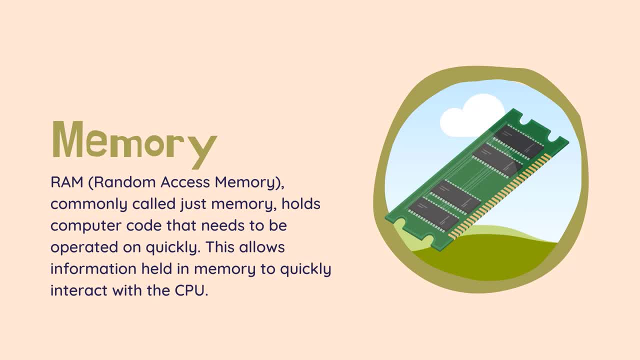 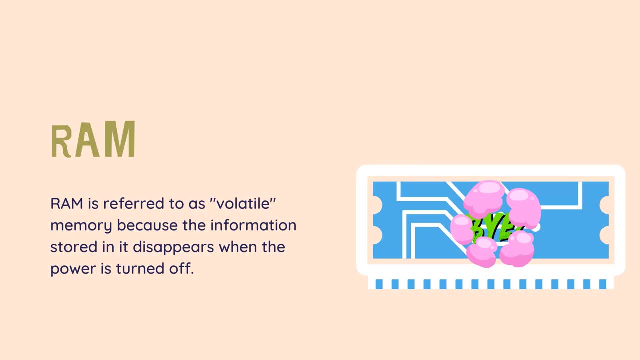 refilled. Don't worry, all computers do this automatically. RAM is just one part of the computer that determines your speed. RAM is referred to as volatile memory because the information stored in it disappears when the power is turned off. Hard drives and flash drives, on the other hand, contain non-volatile memory, which is like paper. 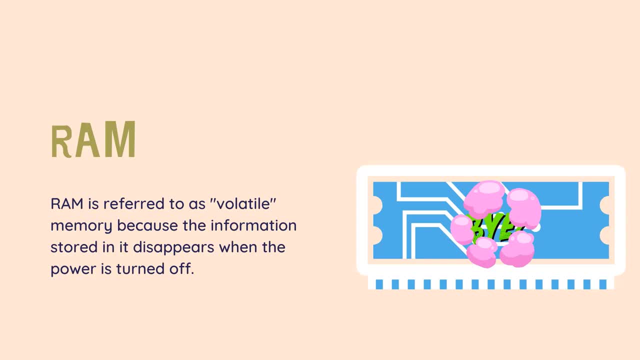 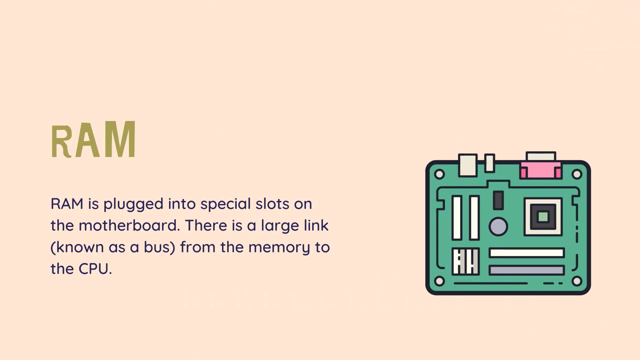 It can be destroyed or erased but when properly taken care of, can last forever. RAM is plugged into special slots on the motherboard. There is a large link, known as a bus, from the memory to the CPU. Each motherboard has a fixed number of slots for RAM. 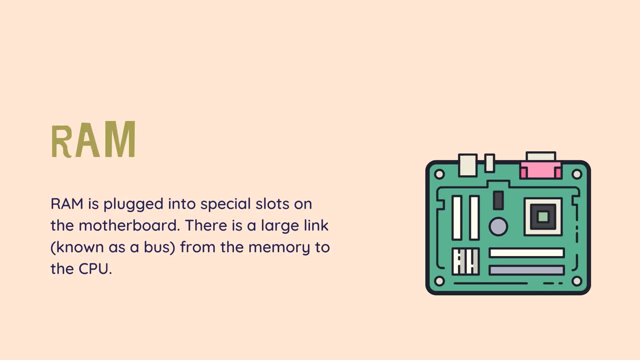 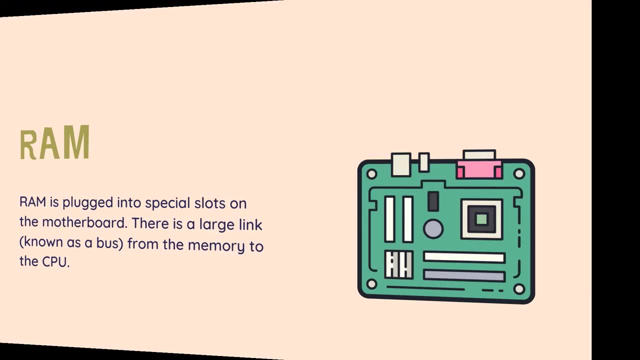 often two or four slots. Only certain types of RAM and sizes of RAM can be used with any motherboard, So before buying check your motherboard details. Hard drive- a partially dismantled RAM can be used to store memory memory or data. Hard drive. 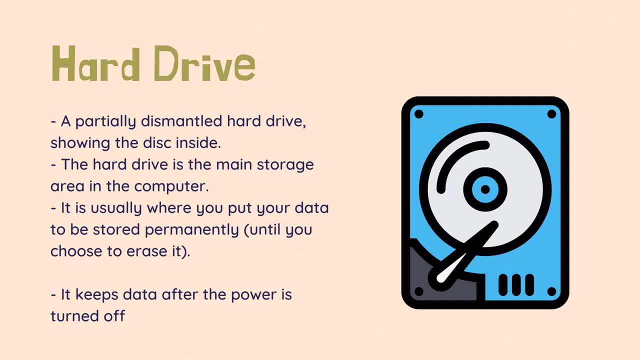 a partially dismantled RAM can be used to store memory memory or data Hard drive. a partially dismantled RAM showing the disk inside Hard drive. a partially dismantled RAM showing the disk inside A hard drive is the main storage area in the computer. It is usually where you put your data. 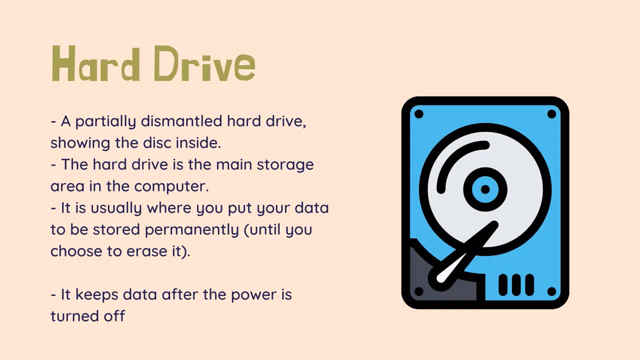 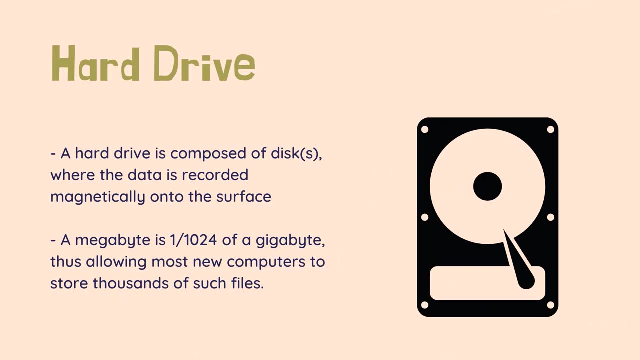 to be stored permanently until you choose to erase it. It keeps data after the power is turned off. The official name for a hard disk is Hard Disk Drive, but is almost always referred to as Hard Drive. Virtually all of your data is stored on your hard drive. A hard drive is composed of. 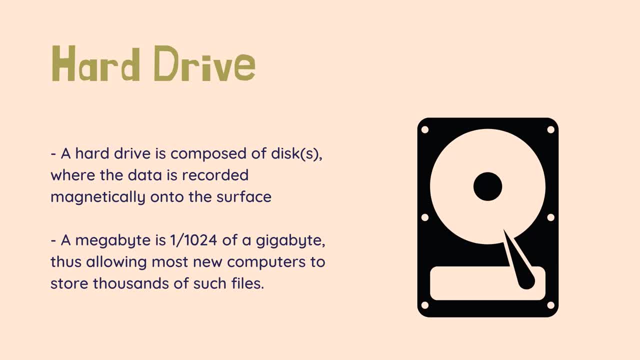 disks where the data is recorded magnetically onto the surface, similar to records, CDs and DVDs. the size of the hard drive today's are usually in gigabytes- is determined by how dense, small the recording is. many of today's major programs, such as games and media, creating and editing programs like 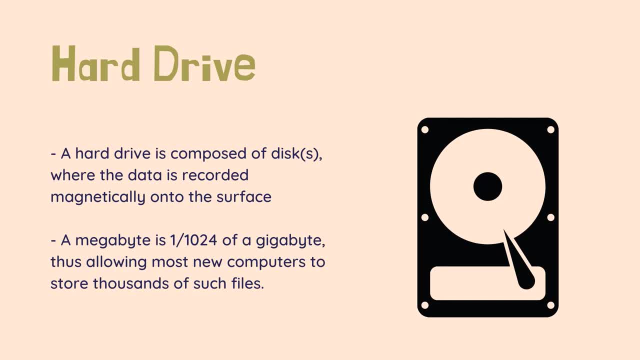 Photoshop and files such as pictures, music or video use a considerable amount of space. most low-end computers as of 2011 are shipped with a 160 gigabytes gigabyte or larger hard drive. in 2019, it is common to find desktop computers and laptops with 1,000 gigabytes, 1 terabyte hard drive or more, as an example an. 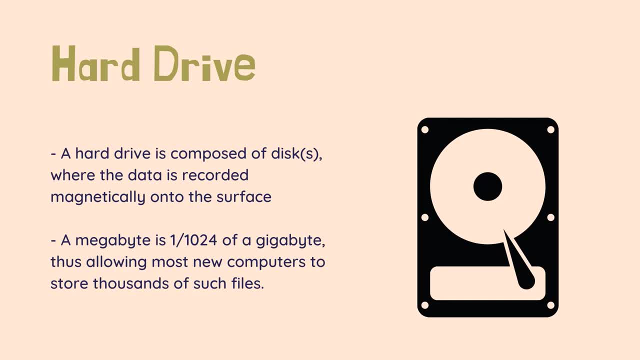 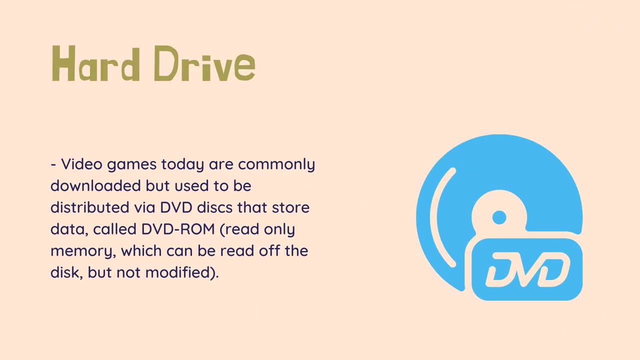 average mp3 file takes between 7.5 and 15 megabytes megabytes of space. a megabyte is one one-third of a megabyte of space, thus allowing most new computers to store thousands of such files. users who wish to store a lot of media on a computer will want a larger hard. 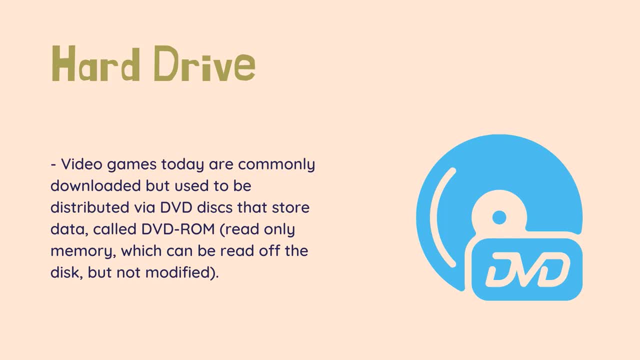 drive, as will users who want to store numerous large programs like modern games or videos, which both require a lot of space. a full-size film is over 4 gigabytes. video games today are commonly downloaded and used on the Internet. this is the reason why computer games are all under the 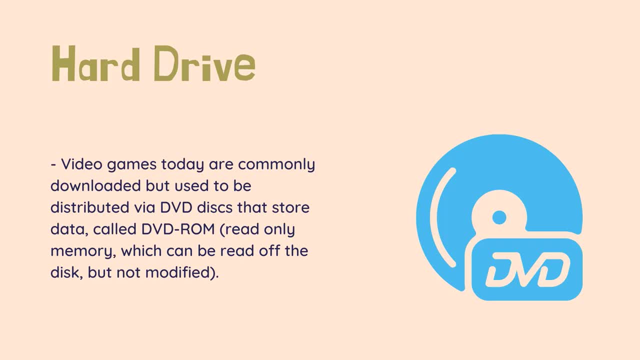 but used to be distributed via DVD discs that store data called DVD-ROM, which can be read off the disc but not modified. A DVD can be anywhere from 4.7 GB for a single-layer disc to 8.5 GB for a double-layered disc. 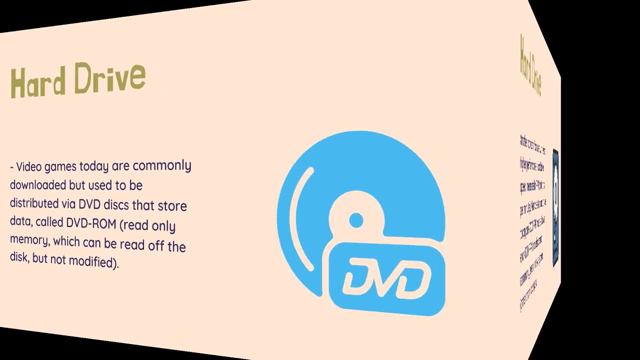 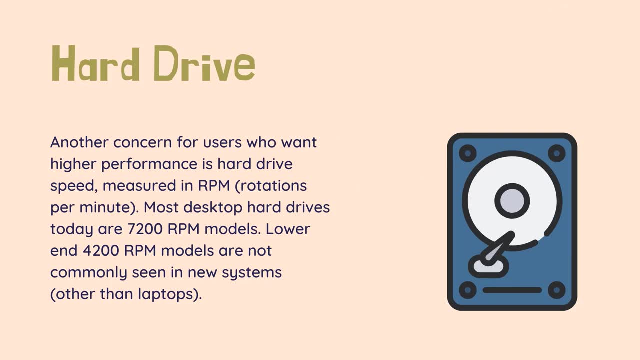 and many large programs are already taking up more than one disc. Another concern for users who want higher performance is hard drive speed measured in RPM. Most desktop hard drives today are 7,200 RPM models. Lower-end 4,200 RPM models are not commonly seen in new systems other than laptops. 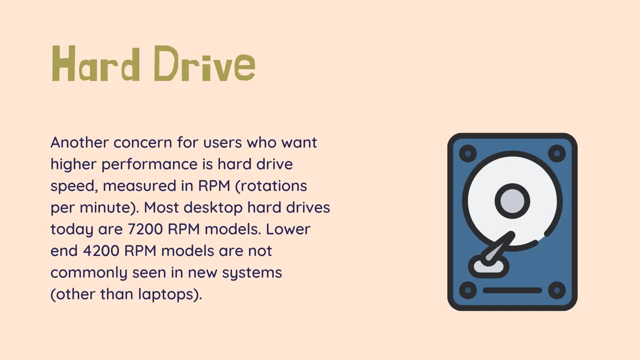 Higher-end 10,000 RPM hard drives are generally seen only in gaming and other extremely high-performance computers, due to their cost. For example, a 1TB 7,200 RPM drive costs around $1,000.. While a 1TB 10,000 RPM drive costs $120 or more. 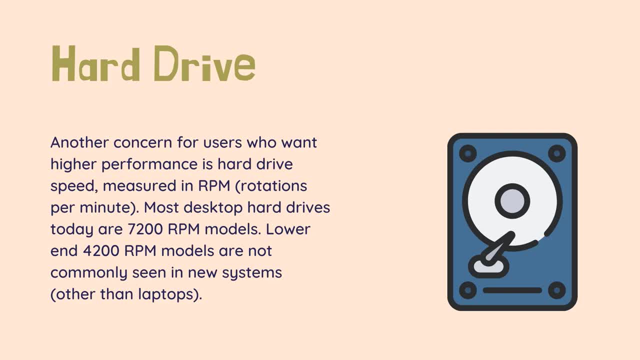 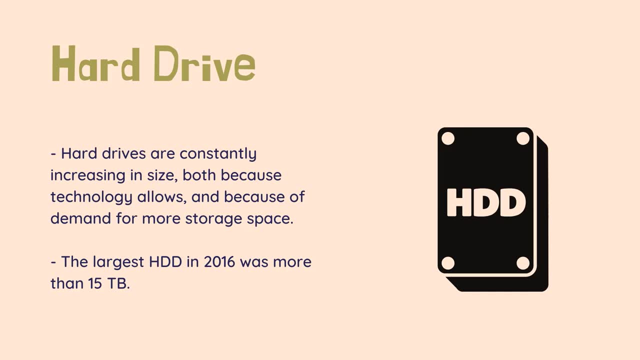 A 1TB SSD starts at about $250.. Hard drives are constantly increasing in size, both because technology allows and because of demand for more storage space. For example, an Apple iMac in the late 90s shipped with a 4GB hard drive. 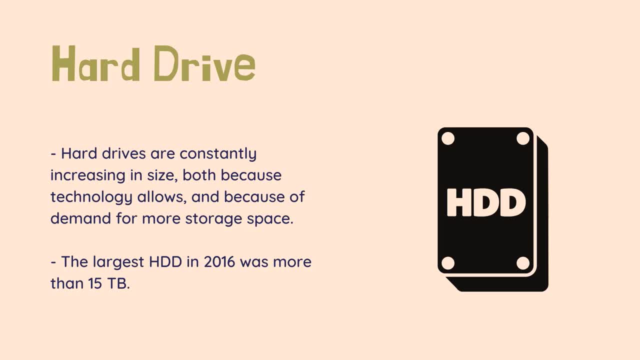 and sold for $1,300, although it should be noted that the cost alone is not indicative of the hard drive, or vice versa. A modern iMac sells for $1,000 and carries a 1TB hard drive with a 21-inch screen and faster processor. 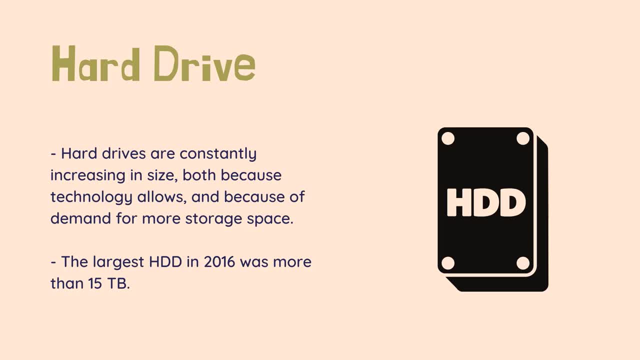 Compare to the original IBM PC, which carried only a 10MB hard drive or 10 1,024 GB. The largest HDD in 2016 was more than 15TB. Many computers already have more than 2TB and, within decades, petabytes, thousands of terabytes. 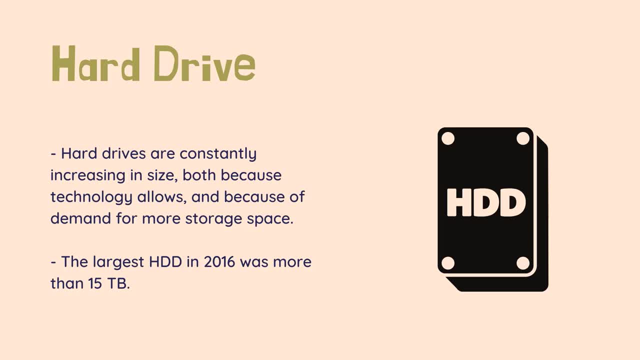 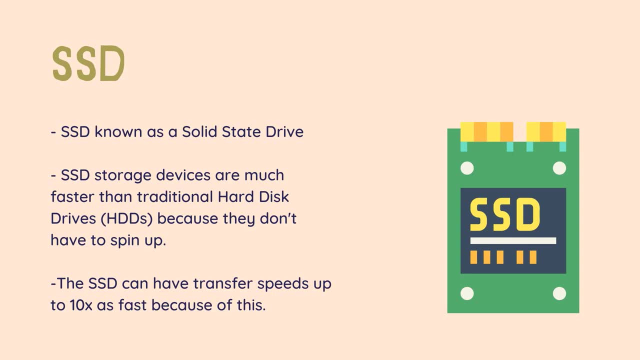 and even exobytes will not be unheard of SSD. the SSD, or otherwise known as a solid-state drive, is a storage device using RAM modules instead of a spinning disk. It is like a hard disk drive, but these storage devices are much faster than traditional hard disk drives. 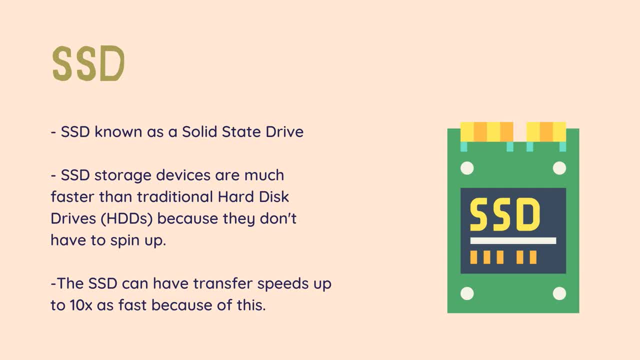 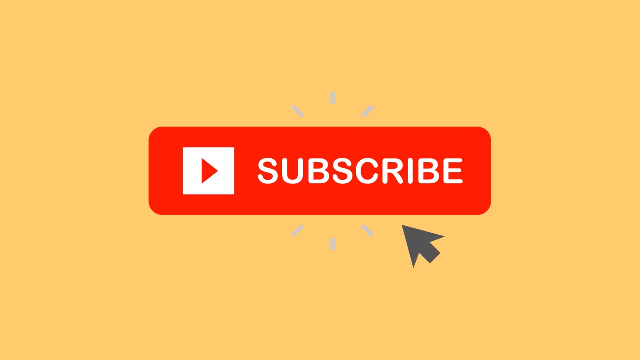 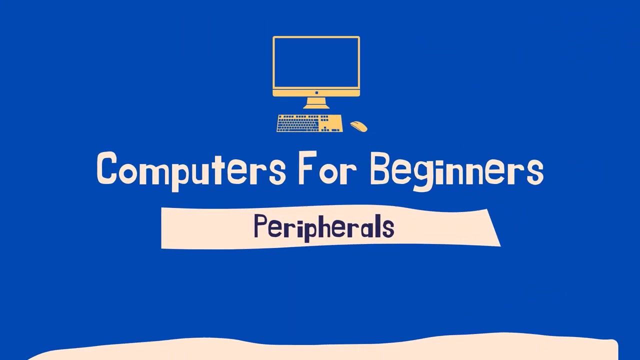 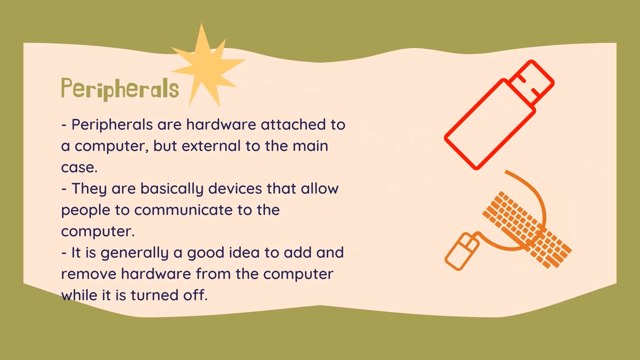 because they don't have to spin up. The SSD can have transfer speeds up to 10x as fast. because of this They are quieter and more expensive than HDDs. undocumented and Studios peripherals are hardware attached to a computer but external to the main case that houses the CPU, hard drives and other such equipment. 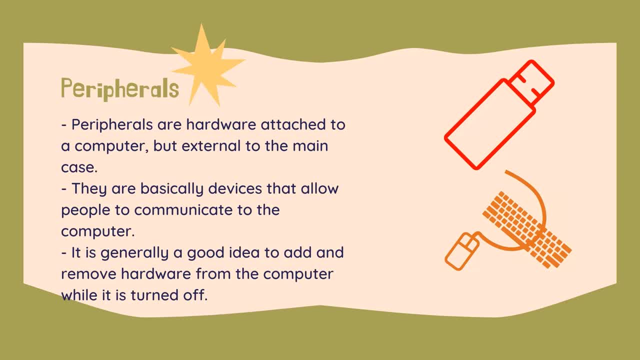 they are basically devices that allow people to communicate to the computer. It isGenerally a good idea, although not as important as it used to be, to add and remove hardware from the computer context while it is turned off. Things such as USB storage devices and keyboards, mice, can generally be inserted and removed. 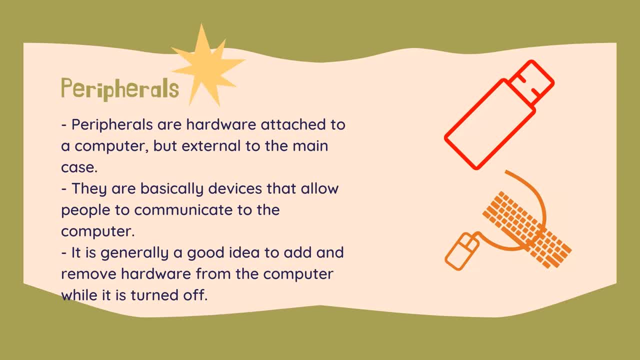 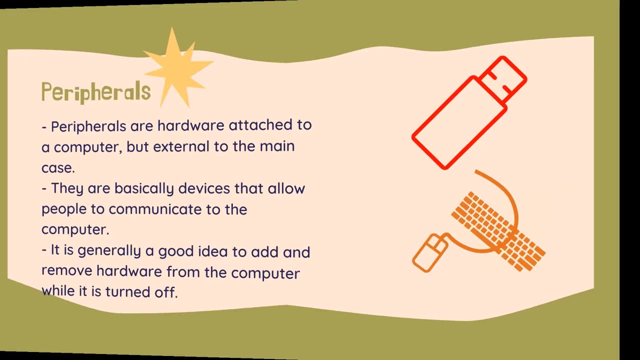 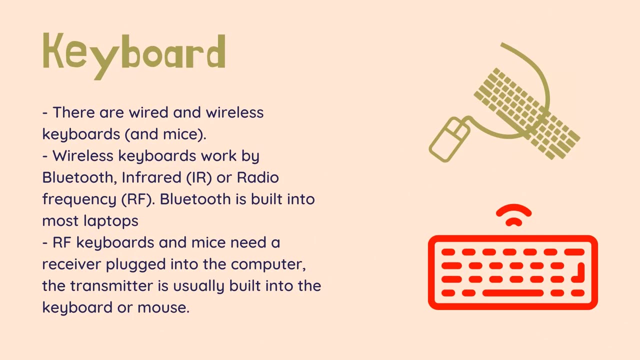 at a whim, with no consequence. however, more advanced things such as printers should be installed according to the manufacturer's instructions, which may include shutting down your computer. There are wired and wireless keyboards and mice. Wired keyboards usually plug into a USB slot. 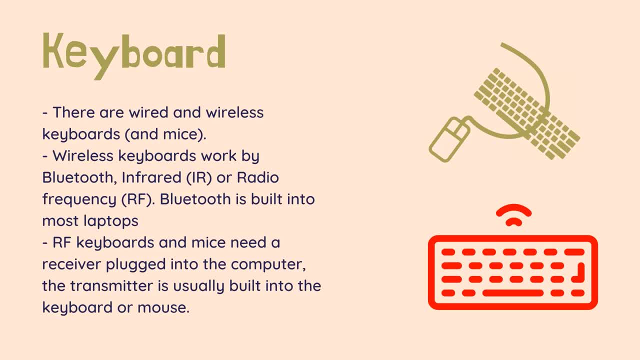 Older style keyboards use the PS2 socket at the back of a desktop. PS2 to USB adapters are available. Wireless keyboards work by Bluetooth, infrared or radio frequency. Bluetooth is built into most laptops, so a Bluetooth keyboard or mouse can connect with no extra equipment. 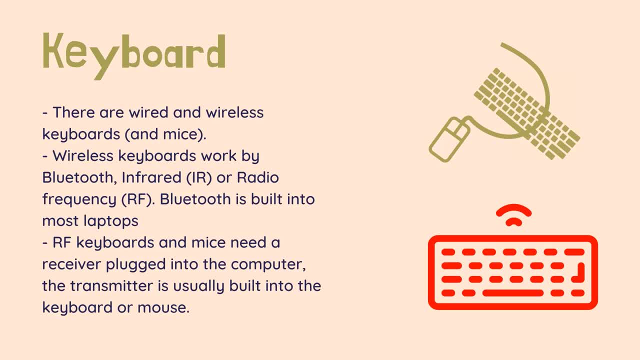 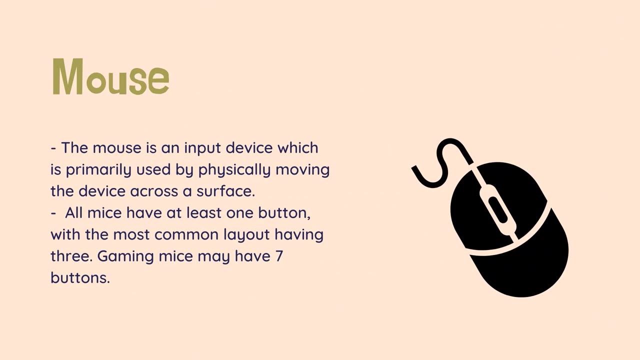 Most desktops do not have Bluetooth built in, but a USB Bluetooth key can be used to add it. RF keyboards and mice need a receiver plugged into the computer. the transmitter is usually built into the keyboard or mouse. The mouse is an input device which is primarily used by physically moving the device across. 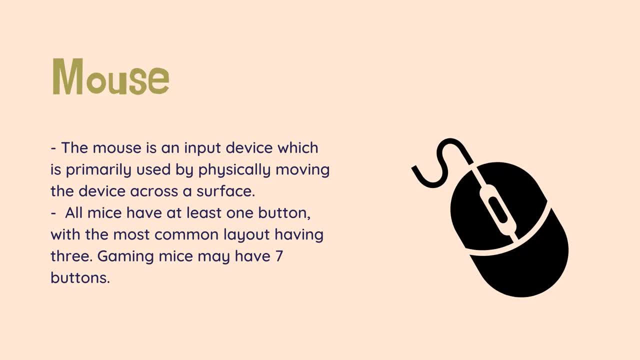 a surface. This causes a pointer symbol called a cursor to move across the screen. The other input comes from pressing a button while the cursor is over an object on the monitor, or clicking. All mice have a cursor. All mice have a cursor. 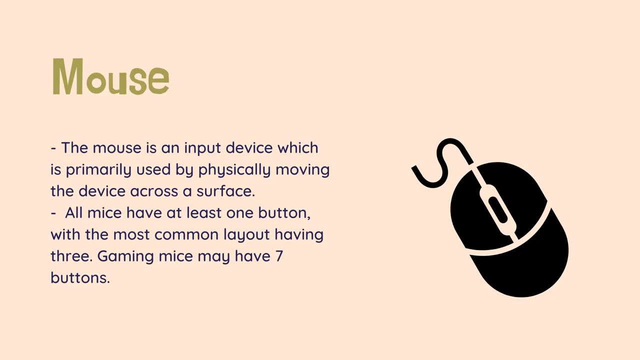 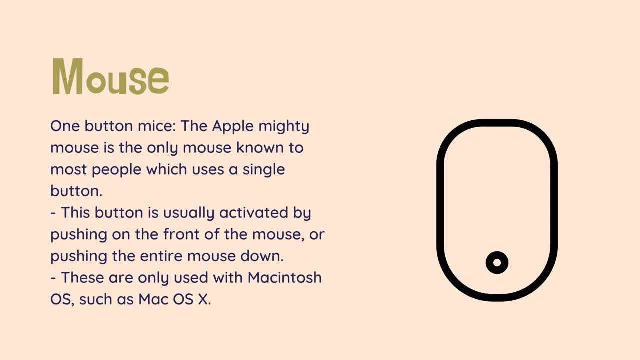 All mice have a mouse button. All mice have a mouse button. Self-mode mice have one mouse button as well. Self-mode mice have at least one mouse button, with the most common layout having three. Gaming mice may have seven buttons. One button mice, the Apple mighty mouse, is the only mouse known to most people, which 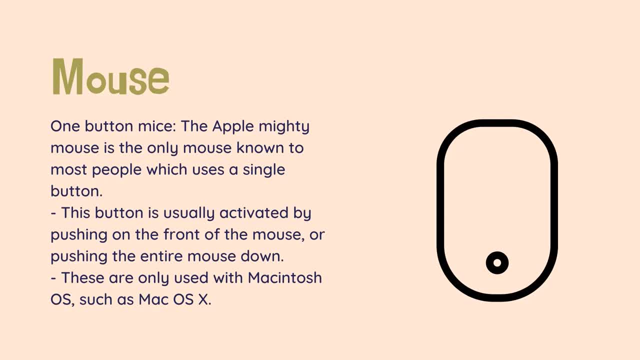 uses a single button. This button is usually activated by pushing on the front of the mouse or pushing the entire mouse down. The right click is done by pressing a control or control key on the keyboard while pressing the main button. 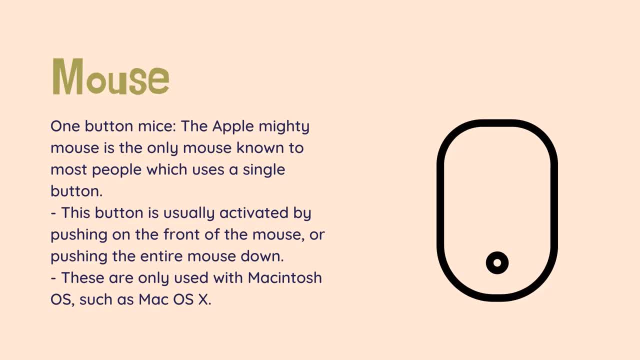 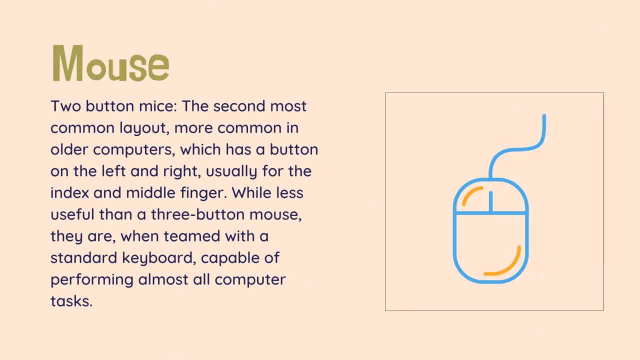 5. used with macintosh os, such as mac os x. two button mice: the second most common layout, more common in older computers, which has a button on the left and right, usually for the index and middle finger. while less useful than a three button mouse, they are when teamed with a standard. 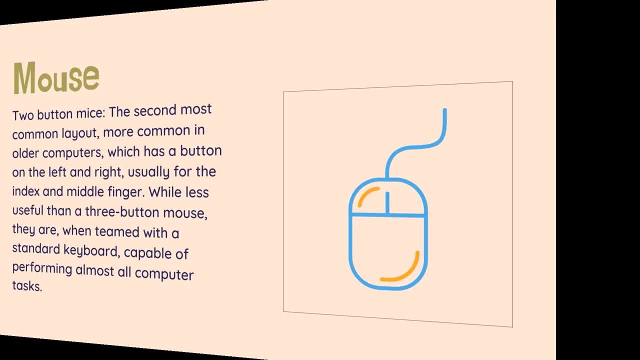 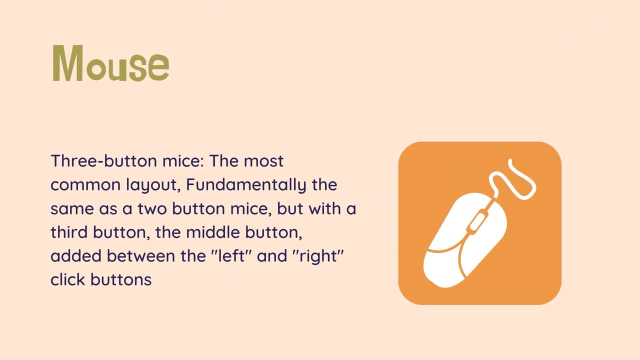 keyboard capable of performing almost all computer tasks. three button mice- the most common layout, fundamentally the same as a two button mice, but with a third button, the middle button, added between the left and right click buttons, while the mouse technically has three buttons. this may be confusing to some users, as the middle center click button is also a scroll wheel. 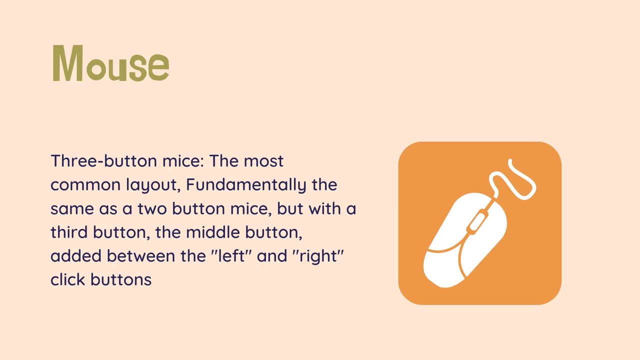 this design allows the user to scroll through documents, make selections and do other tasks by moving a finger. the other way to is to press an arrow key or page up, page down key on a keyboard. the center button can also be press inwards to create a middle click. 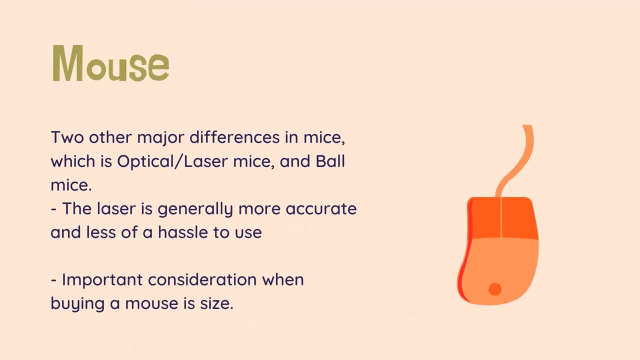 button. there are two other major differences in mice, which is optical laser mice and ball mice. this is how the mouse tells where it is, with the laser measuring the distance it crosses when it is moved and the ball measuring how it rotates. the laser is generally more accurate and less of a hassle to use and can be. 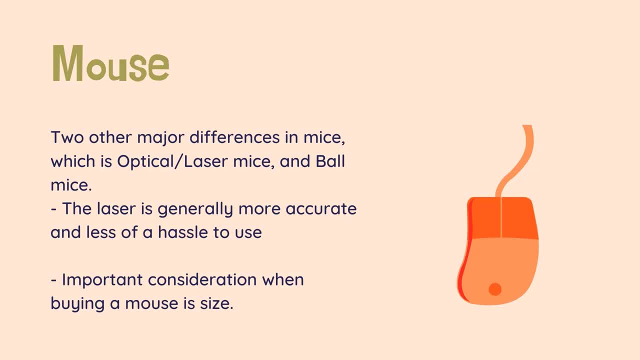 used on more surfaces, but the ball mouse is cheaper. ball mice are rarely seen today. the last important consideration when buying a mouse is size. you should always try to put your hand on a mouse and move it around to see how well it feels in your hand. if it feels awkward- small, big, long or short- look for something better. not only will your 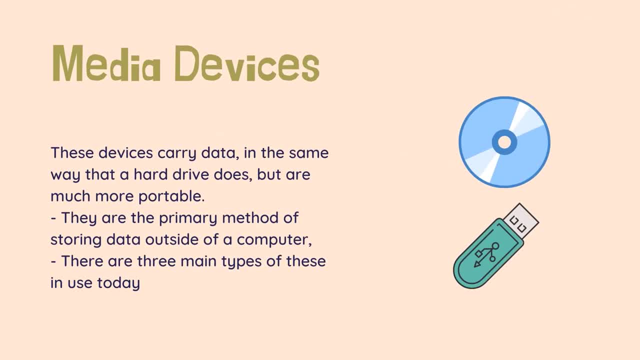 hands. thank you, but you will be more efficient. media devices- cd-rom, dvd, usb- these devices carry data in the same way that a hard drive does, but are much more portable. they are the primary method of storing data outside of a computer and the main method of transferring information between computers without the use of a network such as the internet. 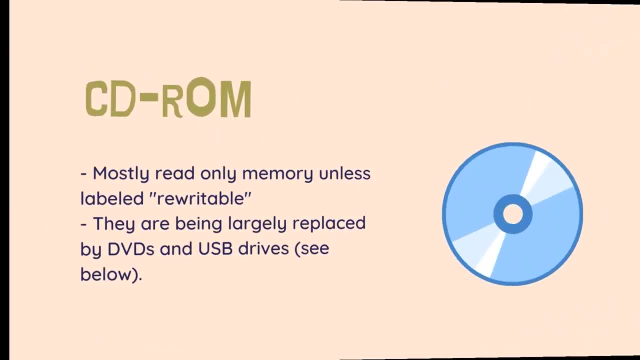 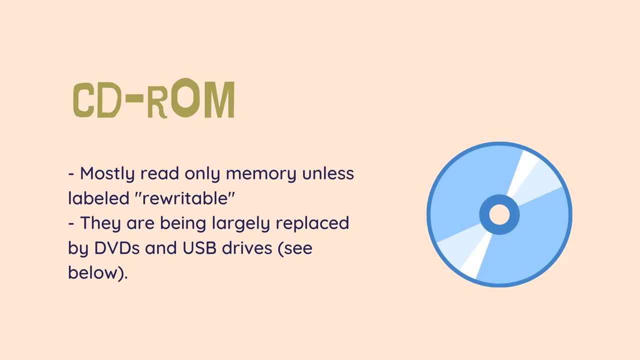 there are three main types of these in use today. cd-rom, mostly read only memory, unless labeled. rewriten, capable of storing 700 megabytes of data. cds have been the most common method of storing data for most of the last decade or so. they are being largely replaced by dvds and usb drives. 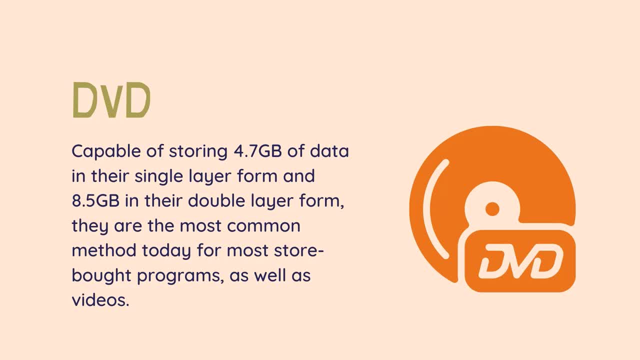 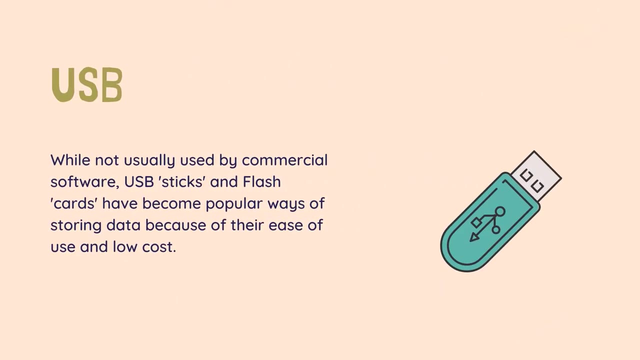 dvd capable of storing 4.7 gigabytes of data in their single layer form and 8.5 gigabytes in their double layer form. they are the most common method today for most store-bought programs, as well as videos, usb flash. while not usually used by commercial software, usb sticks and flash cards have become 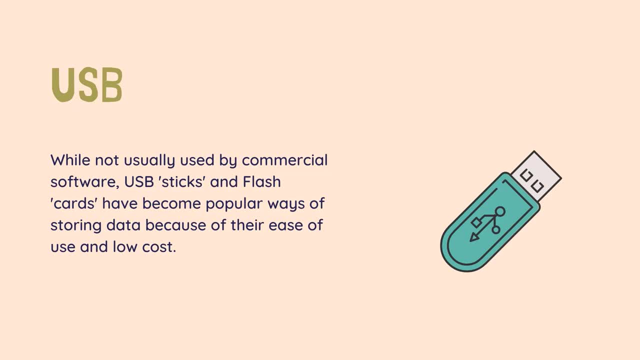 popular ways of storing data because of their ease of use and low cost. while sizes range from 2 gigabytes on old units to 256 gigabytes on larger, more expensive, modern units, the average stick today is four or eight gigabytes, with an average four gigabytes usb stick costing about 15. 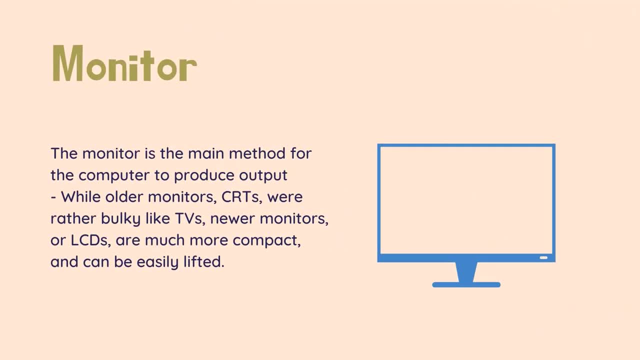 of monde. the floppy disk has been phased out. the monitor is the main method for the computer to produce output. in the same way, a book has pages. a book filled with letters, but in a way you can't possibly understand or even see, is of no use to you. and the same is true for 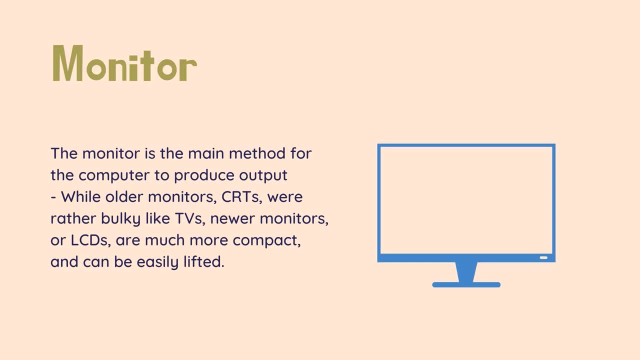 a computer. while older monitors, crt's, were rather bulky, like tvs, newer monitors or lcds are much more compact and can be easily exported to cameras. byputton is a great example of this. yet another way digit但 i have used for a long time compared to follow me and all infos that show me change in the. 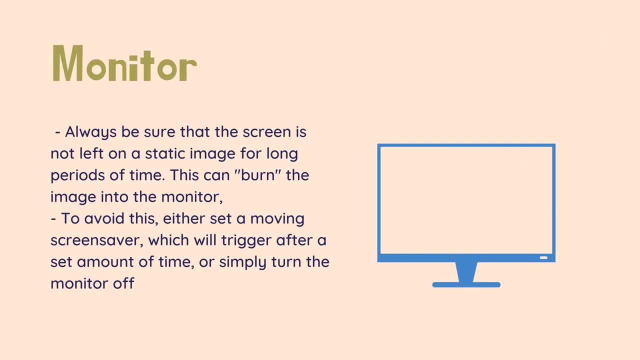 easily lifted. tip to take proper care of your monitor: always be sure that the screen is not left on a static image for long periods of time. this can burn the image into the monitor, meaning that it will have a ghosting effect even when that image is not displayed. this can not only 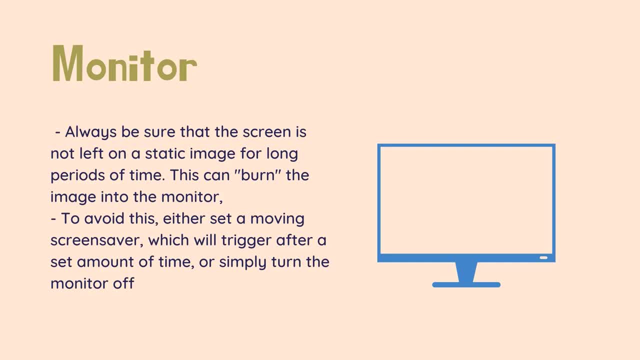 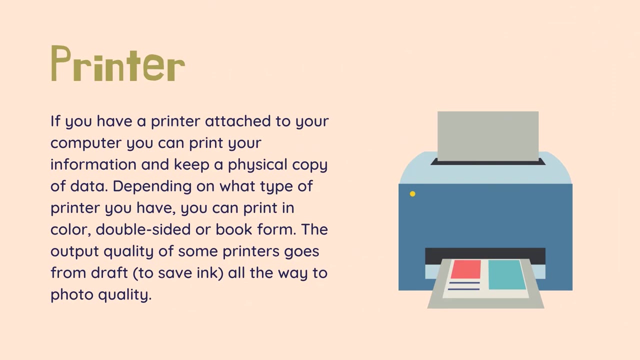 be highly annoying, but in some cases, make it so the monitor needs to be replaced. to avoid this, either set a moving screensaver which will trigger after a set amount of time, or simply turn the monitor off. if you have a printer attached to your computer, you can print your information and keep a. 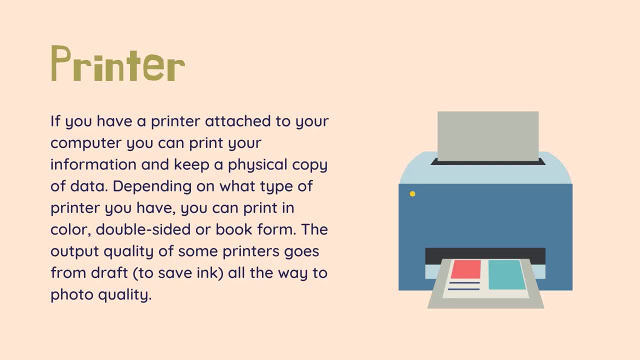 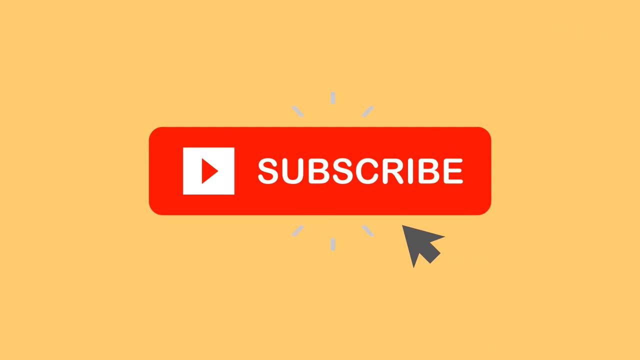 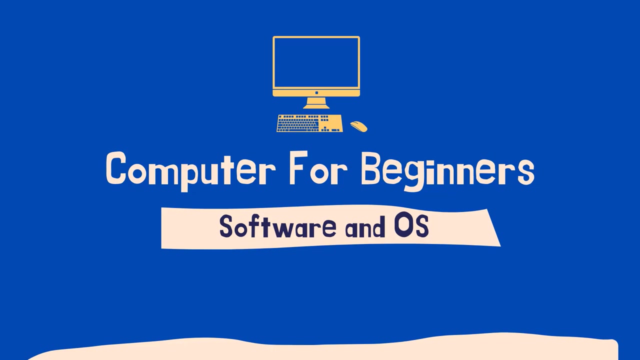 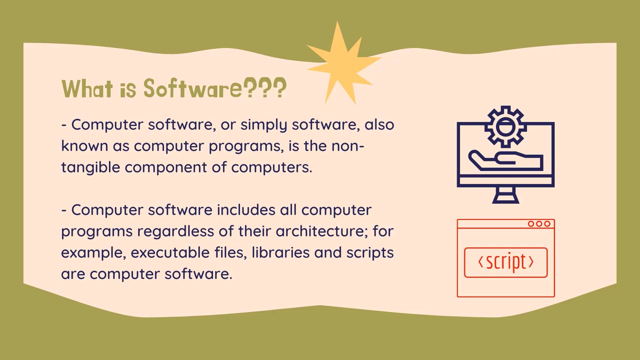 physical copy of data. depending on what type of printer you have, you can print in color, double sided or book form. the output quality of some printers goes from draft to save ink all the way to photo quality. what is software? computer software or simply software, also known as computer programs, is the 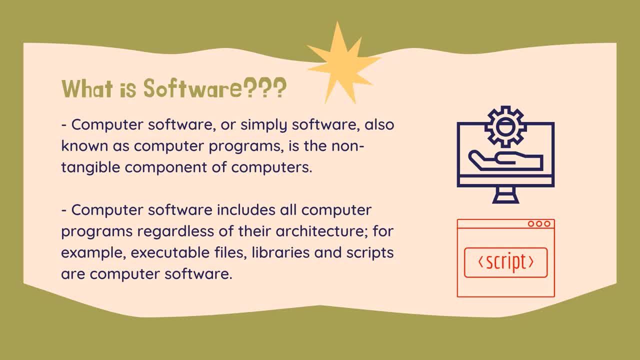 non-tangible component of computers. computer software contrasts with computer hardware, which is the physical component of computers. computer hardware and software require each other and neither can be used in a computer software system realistically used without the other. computer software includes all computer programs, regardless of their architecture. for example, executable files, libraries and scripts are. 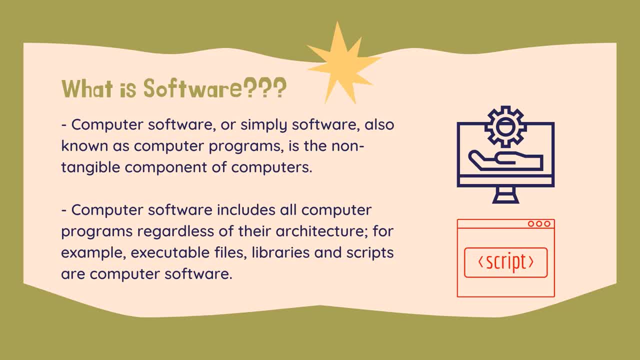 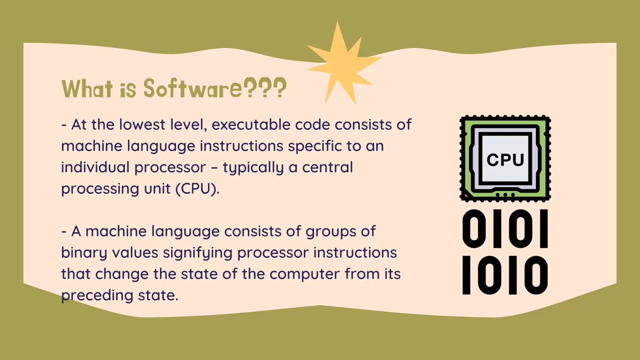 computer software. yet it shares their mutual properties. software consists of clearly defined instructions that, upon execution, instructs hardware to perform the tasks for which it is designed. software is stored in computer memory and cannot be touched at the lowest level. executable code consists of machine language instructions specific to an individual processor, typically a central processing unit, cpu. a machine language consists of groups of binary. 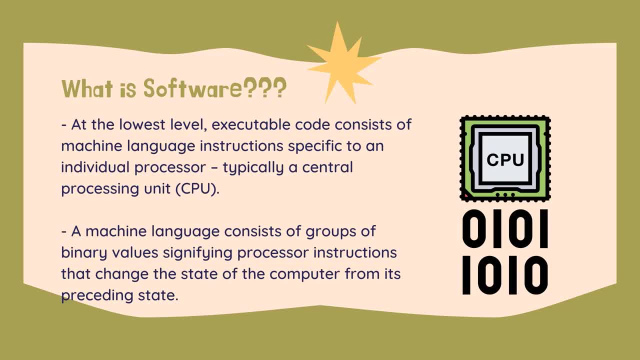 values signifying processor instructions that change the state of the computer from its preceding state. for example, an instruction may change the value stored in a particular storage location inside the computer, an effect that is not directly observable to the user. an instruction may also indirectly cause something to appear. 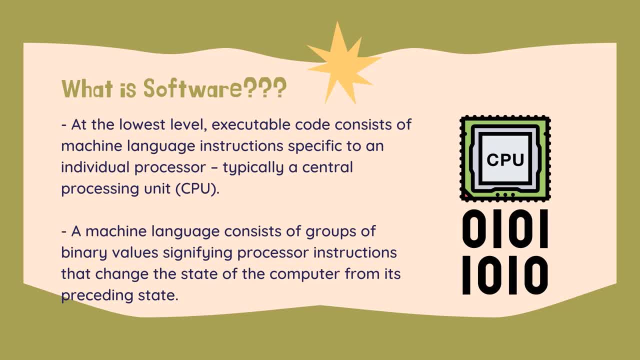 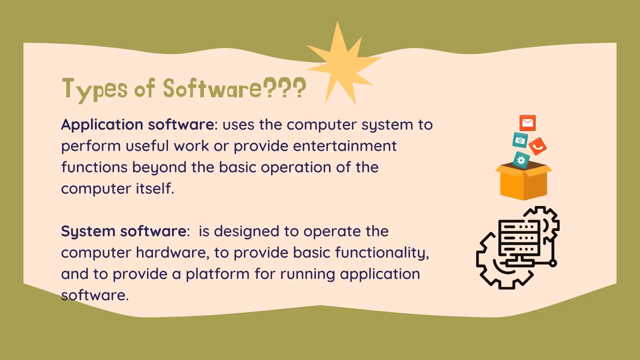 on a display of the computer system a state change which should be visible to the user. the processor carries out the instructions in the order they are provided, unless it is instructed to jump to a different instruction or interrupted application software uses the computer system to perform useful work or provide entertainment functions beyond the basic operation of the 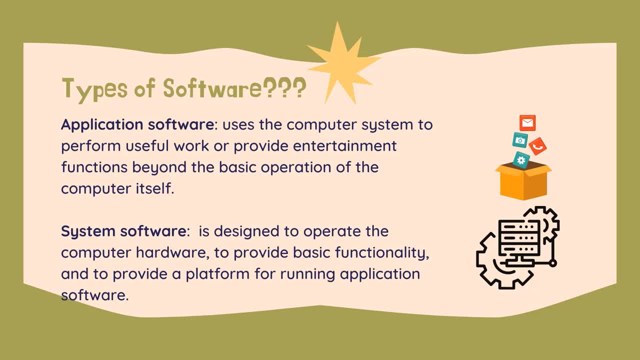 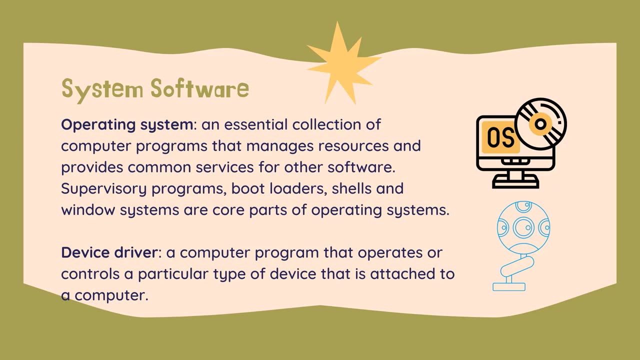 computer itself. system software is designed to operate the computer hardware, to provide basic functionality and to provide a platform for running application. software. system software includes operating system, an essential collection of computer programs that manages resources and provides common services for other software. supervisory programs, bootloaders, shells and windows systems are core parts of operating systems. 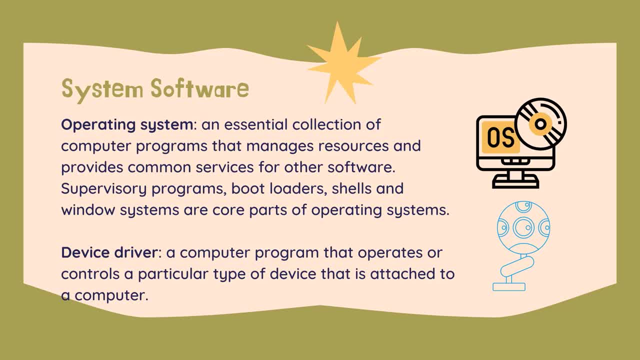 in practice, an operating system comes bundled with additional software, including application software, so that a user can potentially do some work with a computer that only has an operating system. device driver, a computer program that operates or controls a particular type of device that is attached to a computer. each device needs at least. 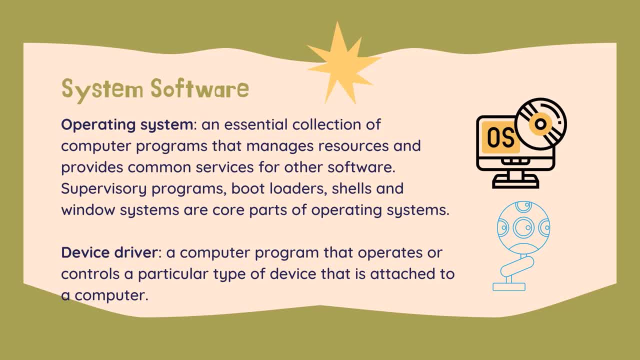 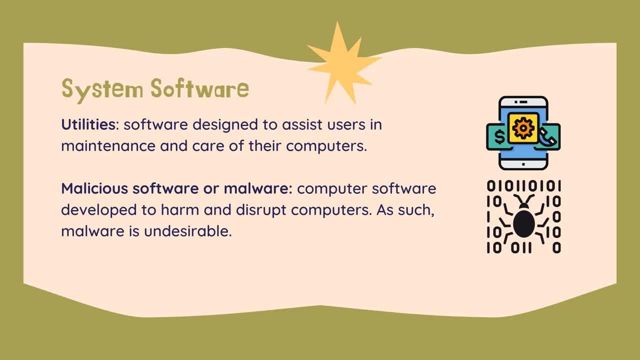 one core responding device driver. Thus, a computer needs more than one device driver. Utilities software designed to assist users in maintenance and care of their computers. Malicious software or malware: computer software developed to harm and disrupt computers. As such, malware is undesirable. Malware is closely associated with computer related crimes. 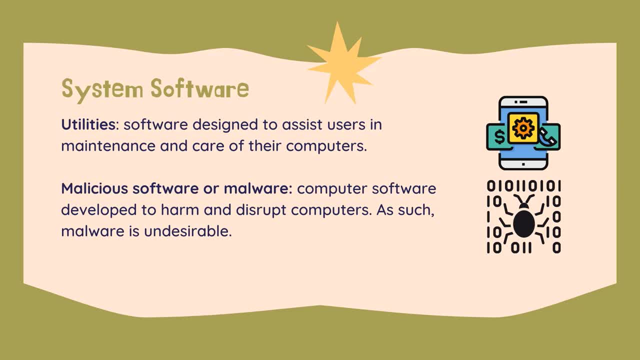 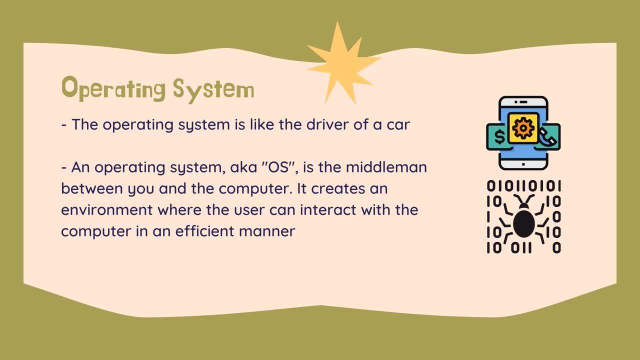 though some malicious programs may have been designed as practical jokes. Operating systems: the major software application on a computer is called the operating system. The operating system is like the driver of a car. While it might seem like it's only telling the car computer what to do, it is in fact also interfacing with the different parts of it. 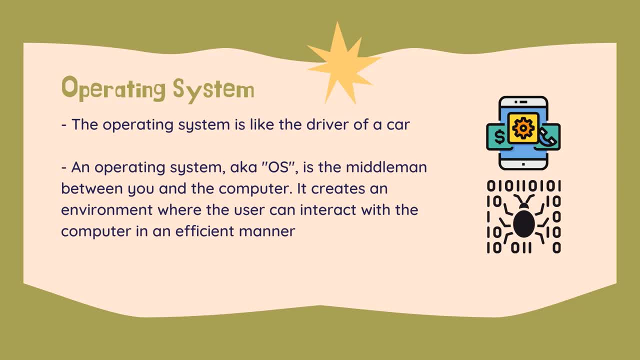 as well as taking any new input, say a map or instructions on where to go, which equate the operating system to a computer. The operating system is a system that is to other software and performing these tasks to the best of its ability. 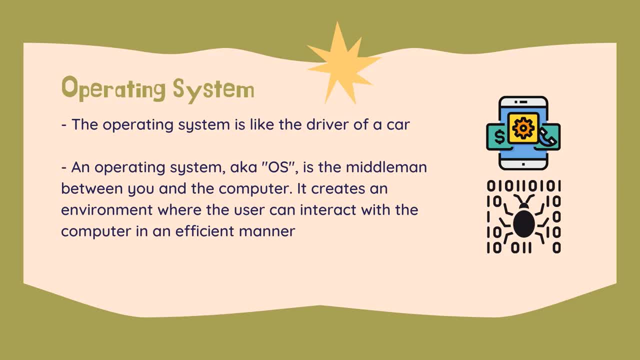 Although many things are compatible across platforms, more involved programs such as photo editing tools and games will not work across all platforms, in the same way that if you started giving your cab driver directions in French, he'd probably tell you to get out, unless you were, of course, in France. an operating system. 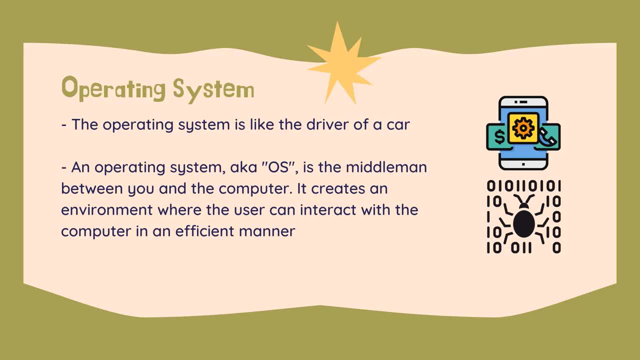 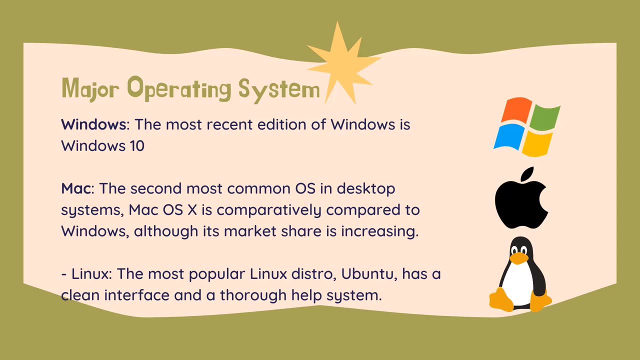 aka OS is the middleman between you and the computer. It creates an environment where the user can interact with the computer in an efficient manner. There are three major OS that you should consider using for your first desktop notebook PC.